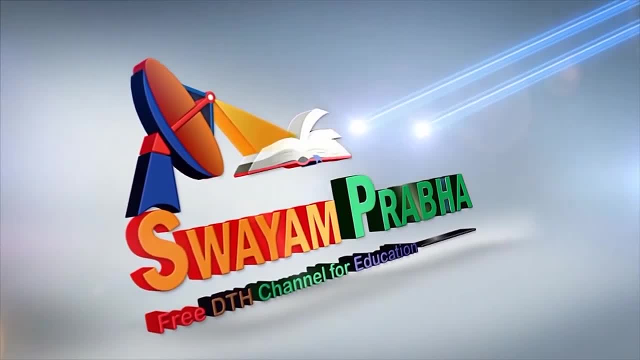 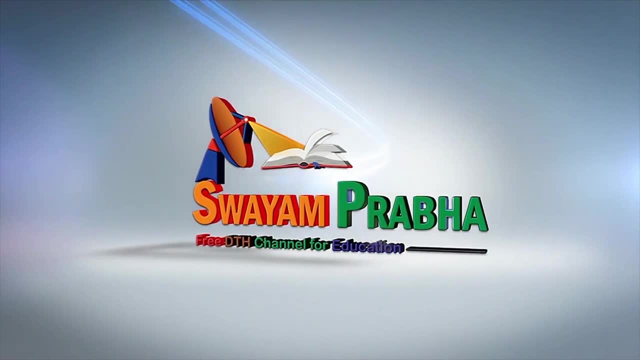 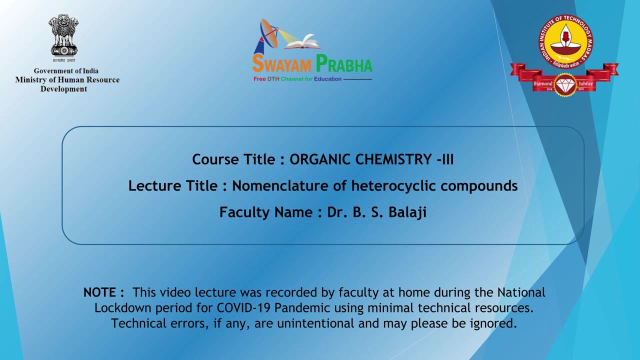 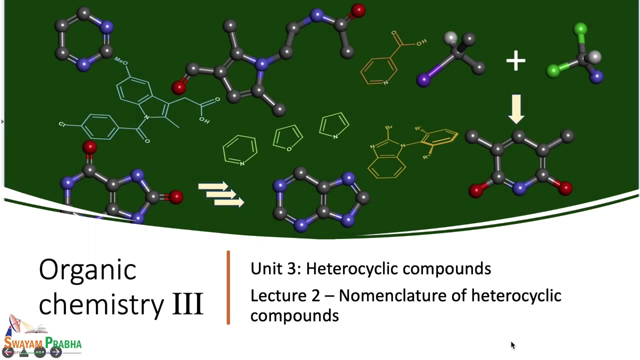 Welcome to organic chemistry, paper 3.. In unit 3, we are studying about heterocyclic compounds. In lecture 2, we are going to study about nomenclature of heterocyclic compounds. I am Dr Balaji, currently working as associate professor in the school of biotechnology at 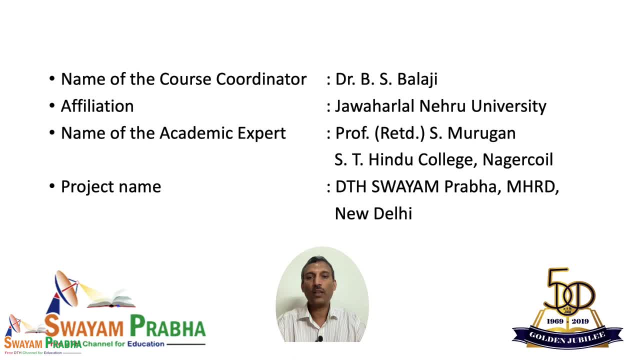 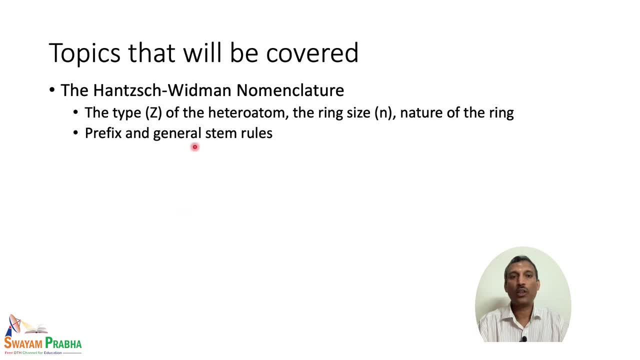 Jawaharlal Nehru University. This project is sponsored by DTH Swaim Prabha, MHRD, New Delhi. The topics that will be covered in this session include the Hans Widmann nomenclature. So we will be studying elaborately, like how heterocyclic compounds are named. We will 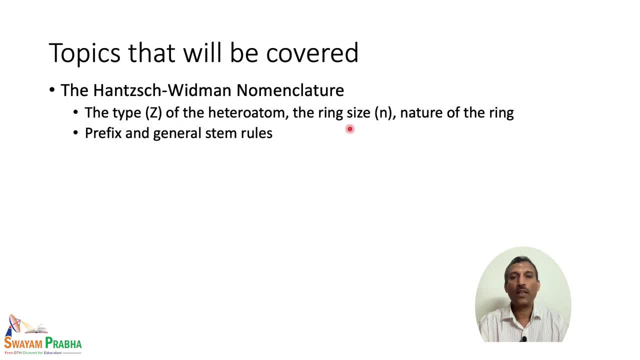 look at the type of the heterocyclic compounds, The heteroatom, the ring size and the nature of ring. So these are all the three important parameters based on which heterocycles are named That we will study. We will also study. 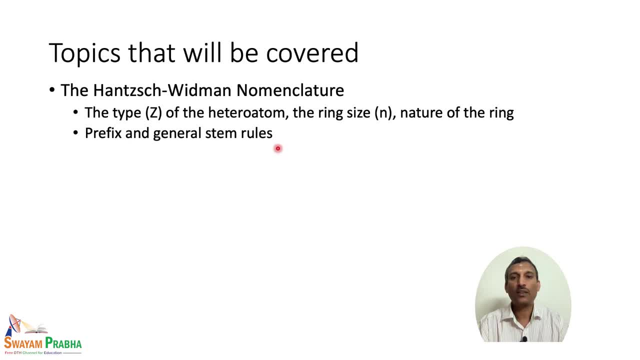 about the prefix and general stem role, Whether it is a saturated system, whether it is an unsaturated system, whether it has a nitrogen oxygen or sulfur heteroatom. How we are going to name that compound we will be studying in this particular session. Let us look at. 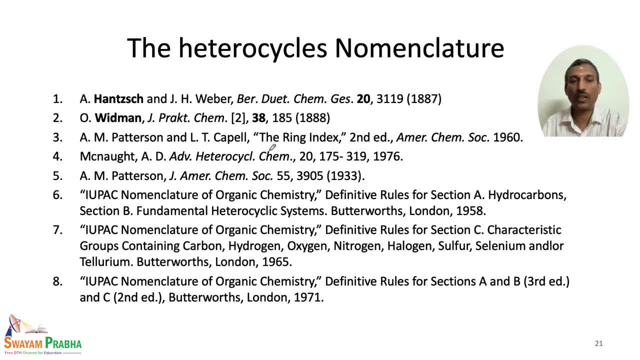 the different nomenclature. So here are various journal articles. names are given, So those who are interested can actually go through many of the papers, although these are very old papers- 1887 and 1888.. So Hans and Widmann are the two great scientists who had introduced the nomenclature for heterocyclic. 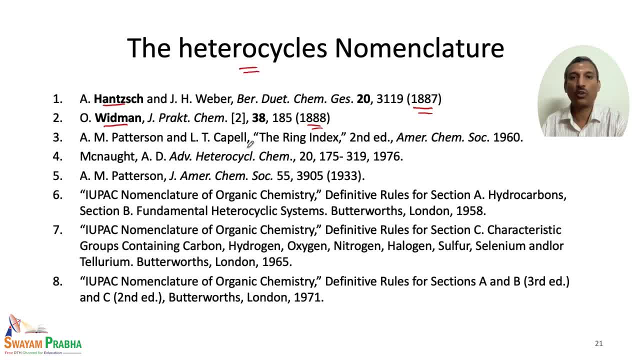 compounds. So that is the reason nomenclature for heterocyclic compounds bears their name. So we have the Hans Widmann nomenclature for heterocyclic compounds and later on IUPAC and other people had actually modified some of the rules and 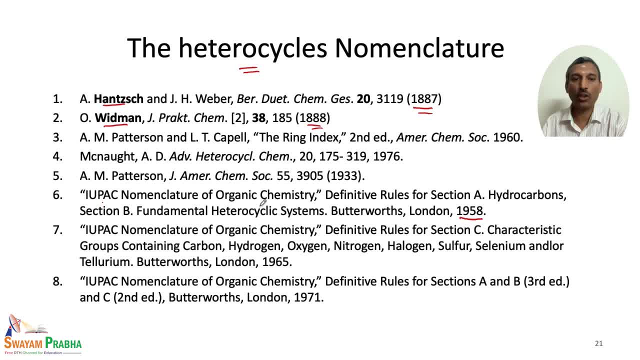 in 1958, they have introduced the IUPAC nomenclature where they have given specific rules for heterocyclic systems, and later on, in 1960 also, they have modified with how to name the compounds when they have oxygen, nitrogen, halogen, sulfur, selenium and artelurium compounds and later. 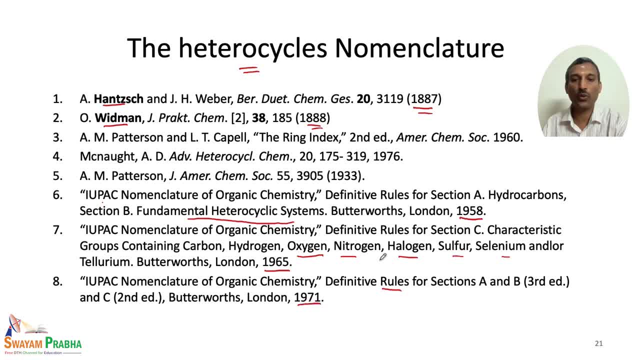 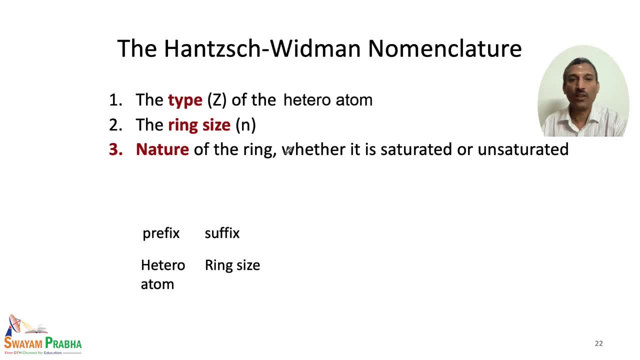 on in 1971. they also have included more sections for the nomenclature for heterocyclic compounds. So according to the Hans Widmann nomenclature rule we have three major rule we have to remember. one is called the type of the heteroatom. 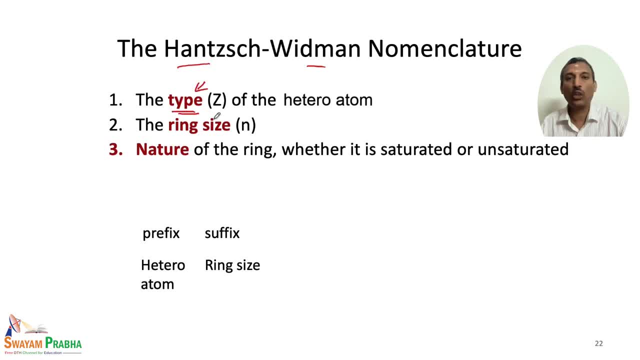 So what is the type of the heteroatom That is being included in the ring? then we talk about the ring size, that is the number, and the third one is the nature of the ring, whether it is a saturated one or unsaturated one. So these are all the three major rules we have to remember while naming a compound, especially. 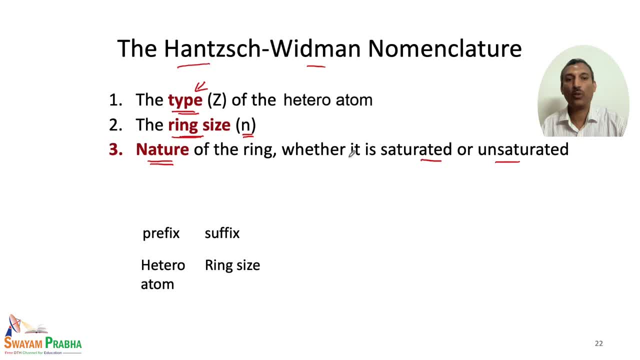 the heterocyclic compound according to Hans Widmann rule. So we have something called the prefix and suffix. we also have heteroatoms, we have ring size. So these are all the important things we have to just keep in mind and once we go through, 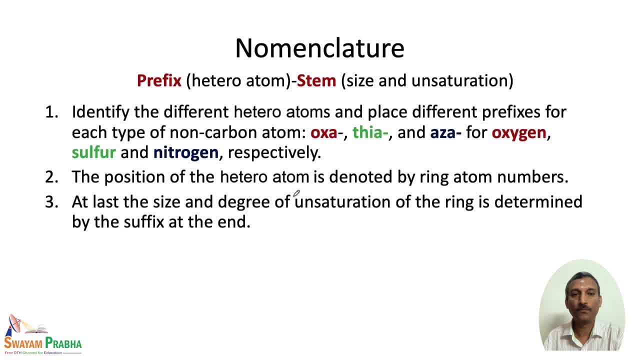 the nomenclature. we can study more about that. So what is the prefix and suffix? So basically, the prefix is basically the heteroatom. whatever is the heteroatom that is given as the prefix, say, for example, for many of the heterocyclic compounds, when oxygen is present. 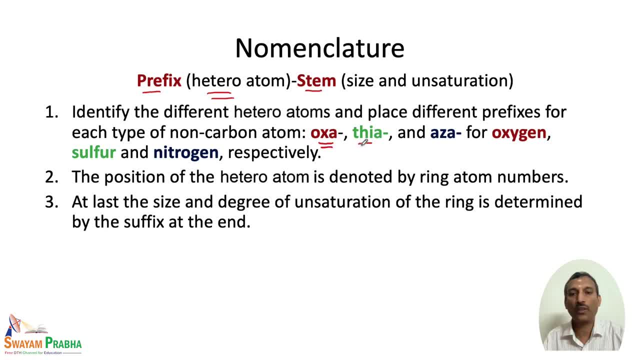 we give the prefix oxo, if sulfur is present, we give the prefix thia, and when nitrogen is present, we give the prefix asa. so these are all the three different prefixes which are actually added to the cyclic nomenclature. so the first one is the prefix we have to know because we are going. 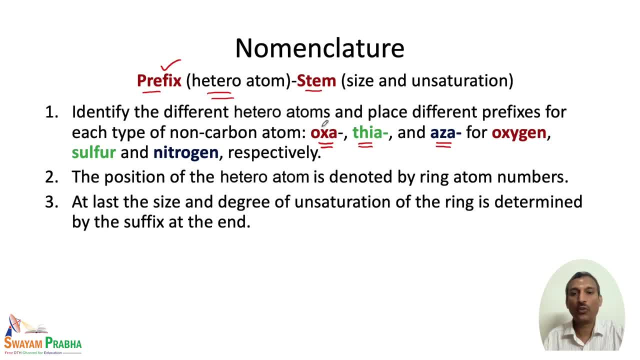 to talk about only oxygen, nitrogen and sulfur. so oxygen is oxa, sulfur is saya and nitrogen is asa and the stem is the second one. that is size and the unsaturation. so these are all the three rules, whatever we saw. that is one is what is the heteroatom? so this is number one and the size. 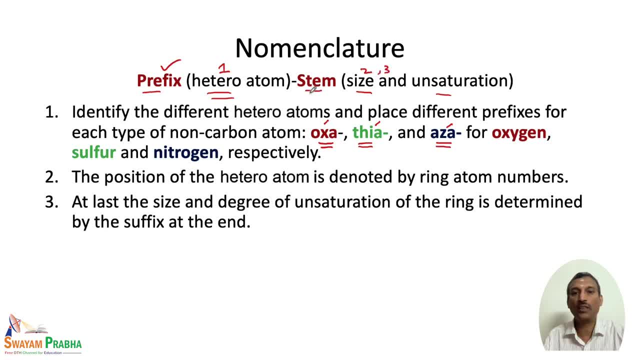 and unsaturation is number two and three. so this is the stem based on which we are actually going to name the compound. so how do we name the compound? basically, the position of the heteroatom is denoted by the ring atom number. so what position the heteroatom is present in most case. 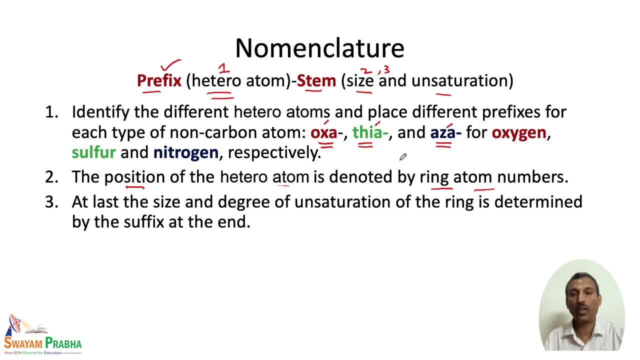 if we have only one heteroatom, then we start with the numbering from the heteroatom. so we have only one heteroatom, then we start with the numbering from the that particular heteroatom only, so it will get the least number, that is one, and then the rest of the. 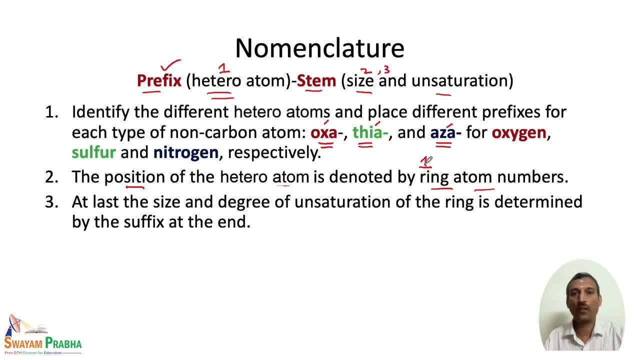 compound is named based on the heteroatom, whatever is present and when the. at last, the size and the degree of unsaturation of the ring is determined by the suffix at the end. so these are all the simple basic rules, and once we apply this, we will understand how to actually name a heterocyclic. 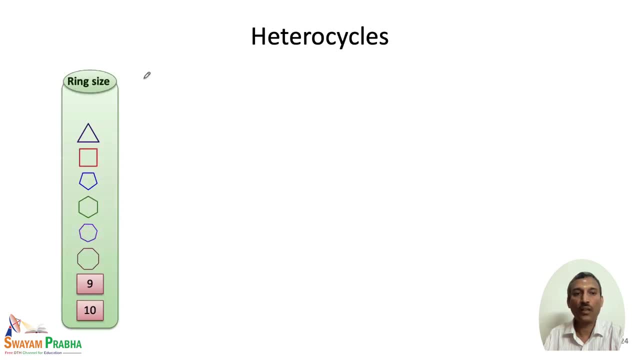 compound, so we have different ring sizes. so this is one of the things we have seen, because we have three major types. one is the heteroatom. what is the type of the heteroatom then? what is the ring size? then we also have whether we have the saturated or unsaturated system. so these are all the three. 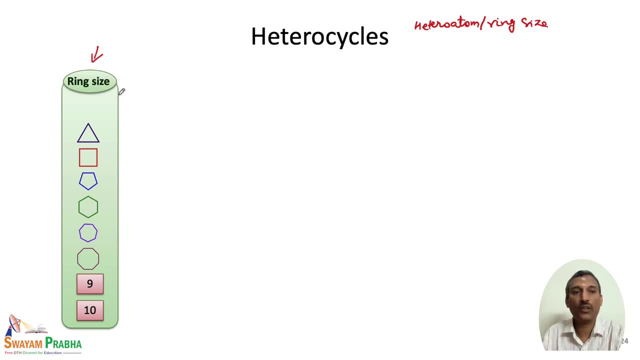 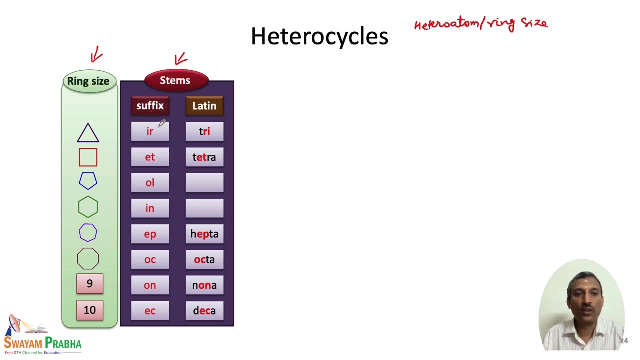 major rules we have to remember, and the first one: we are going with the ring size. so the stem actually is given based on the ring size. so the suffix is actually the one which we actually add to the name. so when we have a three membered ring, it is called ir, so this ir actually came. 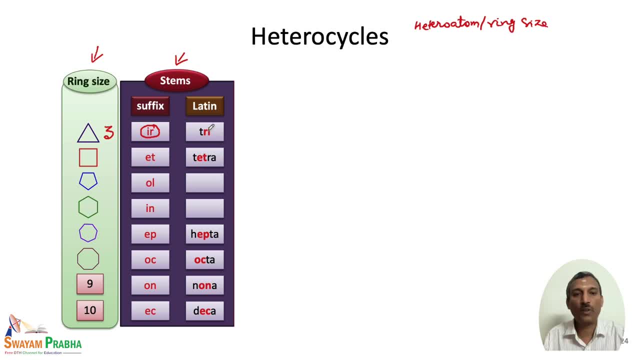 from the latin word try, but it is little bit shifted. that means instead of ri we are actually using it as a ir, and when it is a four membered ring, tetra et is the word and that et is actually used as the suffix. and for the five and the six membered ring. this is quite uncommon and there is 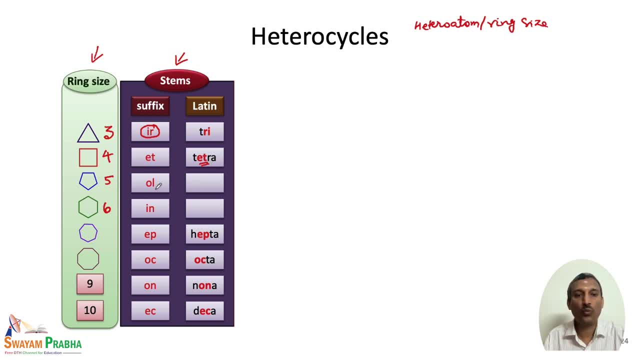 no latin equivalent for this one. generally, ol and in are the names which are added as a suffix in the case of heterocyclic nomenclature and for the other case. in the case of heterocyclic nomenclature and for the other cases, we can directly follow the latin name. so hepta, that means ep, is given. 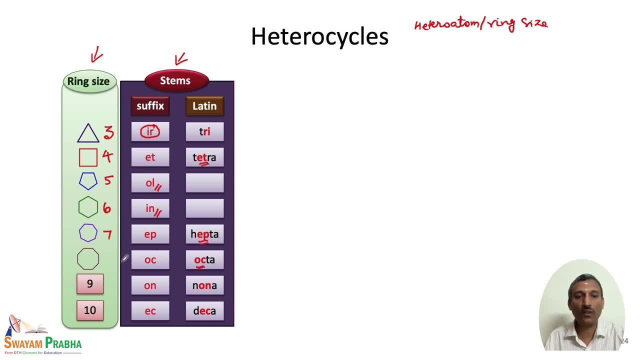 for the seven membered ring. acta oc is given for the eight membered ring. nona on is given for the nine membered ring. deca ec is given for the 10 membered ring. so this is how, from 7, 8, 9, 10, they. 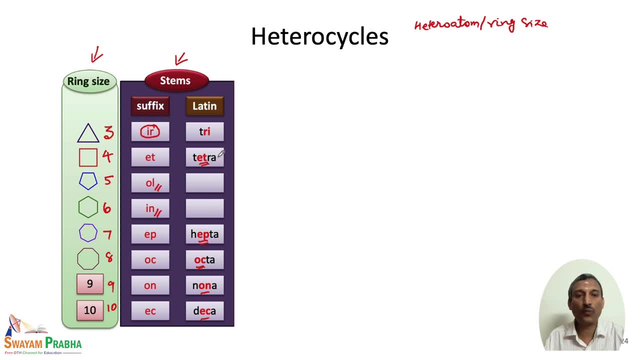 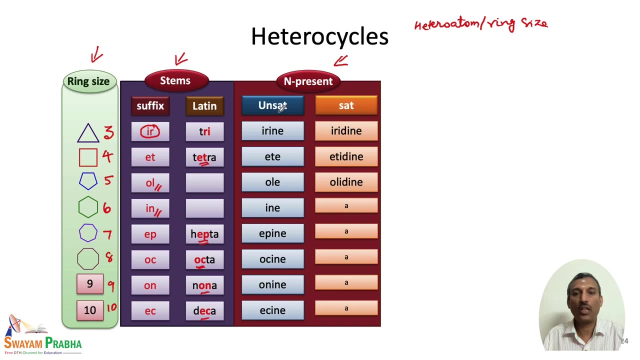 simply followed the latin nomenclature. and even for 4 the latin nomenclature is followed, but 3, 5, 3, ex exceptions to this particular rule and depending on whether nitrogen is present, we actually have a different name. if nitrogen is absent, then the name is little bit different, say: 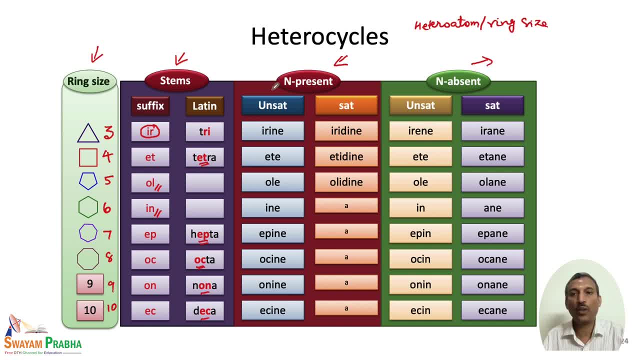 for example, when nitrogen is present, we have two cases, because we also talked about the third rule, where we talk about the saturation and unsaturation. so when the nitrogen is present, we have two types. one is a unsaturated system. we also have a saturated system. so depending on whether the ring is a saturated one, 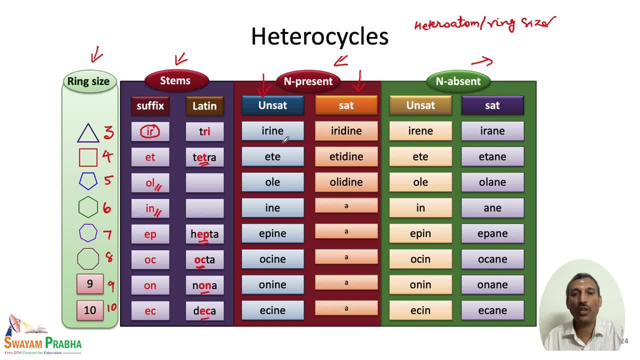 or unsaturated one, the name actually changes. so the suffix, whatever we add, is ir. so if there is a unsaturation, the name will be i r i n? e, and if there is a saturation, instead of ine it is ire di ne. so this id is added extra when it is a saturated one. the same way, if 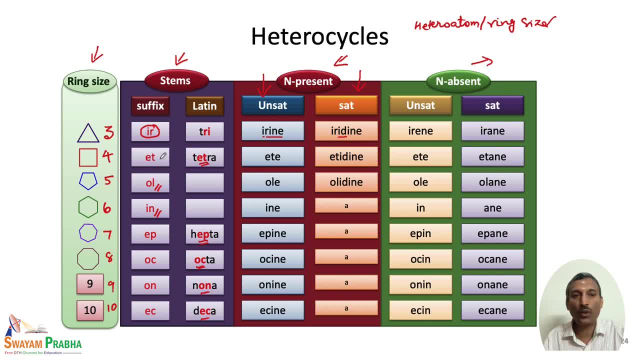 it is unsaturated ring with the four membered ring its name will have ete, whereas when there is a saturated thing instead of ete we else actually have additional things: ettidine. so when we name the compounds we will have will actually see the difference how we have to actually name. but these are all the various 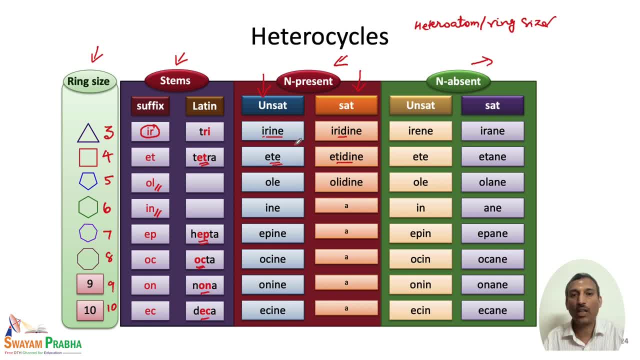 important things we have to remember while we are naming the heterocycle and when we go to the systems. where nitrogen is not there, that means we have only oxygen or sulfur. in that case, the i is not present. instead of i we have e in the case of three membered ring and for four membered. 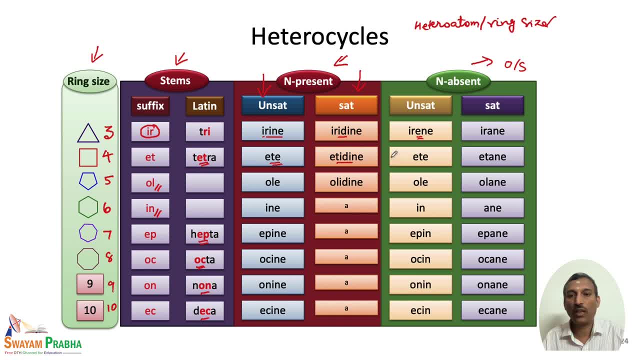 ring and five membered ring. if you look at very carefully whether the nitrogen is present or not present, they have the same stems and the only difference comes in the case of saturated systems, if nitrogen is present. if it is a four membered ring, it will have the ending like etidine and 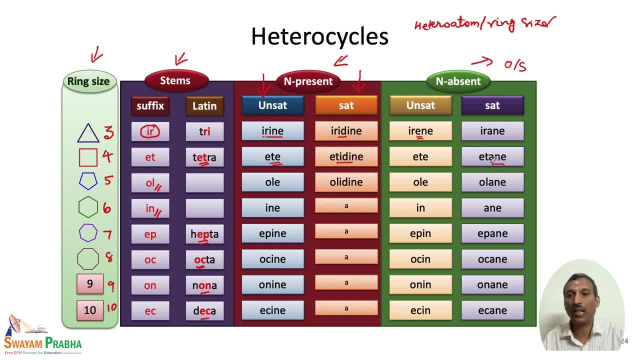 if it is nitrogen is not present, then it will have etain. so that is the only difference for the four membered ring and for the five membered ring, olidine is the ending for the saturated ring with the nitrogen. o lane is the name for saturated system without nitrogen. 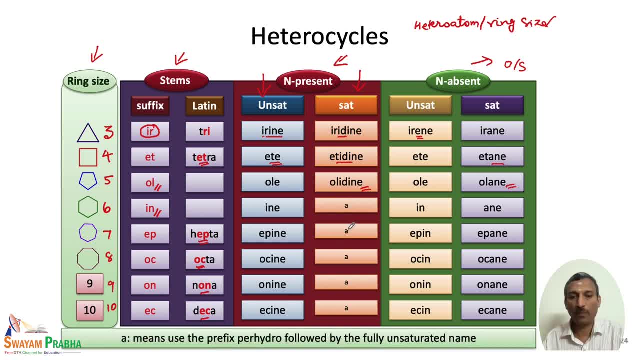 and when we talk about a, here is means the prefix pre-hydro will be added to all the saturated systems. so when the nitrogen is present, we actually add the prefix per hydro to the name. so these are all the by which the heterocycles are named. of course, this rule looks highly complicated and it is very 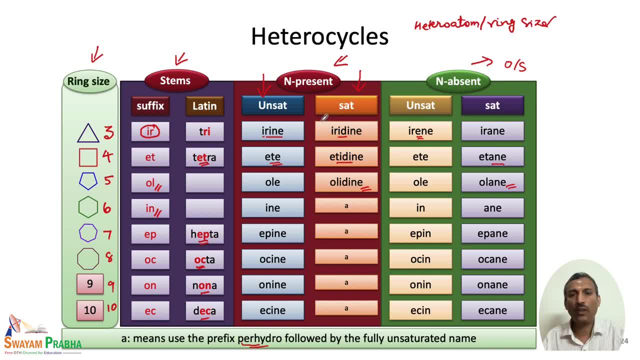 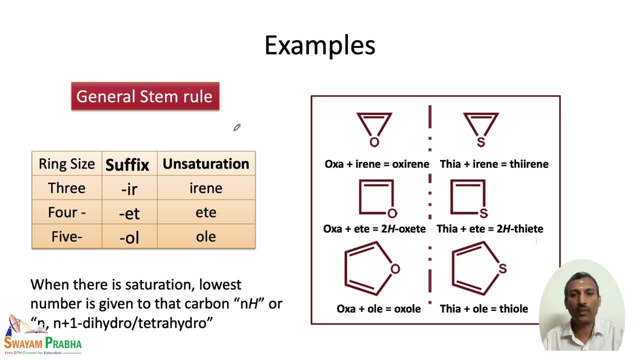 difficult to follow, but but when we use the examples we will exactly know how these rules are actually applied. so let us take the example of the simple system that means oxygen system we are looking at here. so here there is no nitrogen, so that rule is going to be little bit different. 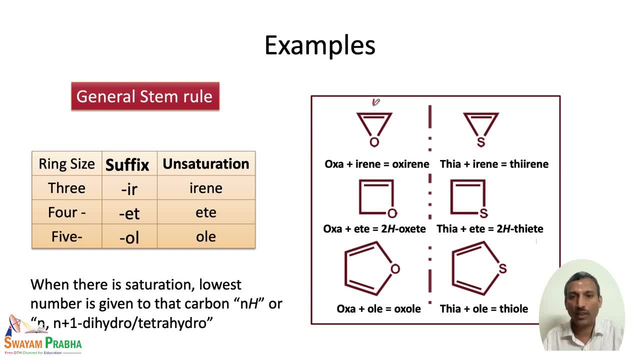 so let us start with the basic rule. so this is a double bond. so this means this is a saturated one, this is unsaturated one. so all the examples given here are due to unsaturation, because we have at least one double bond in the system. so whenever there is one double one, this belongs to unsaturation. so when there is 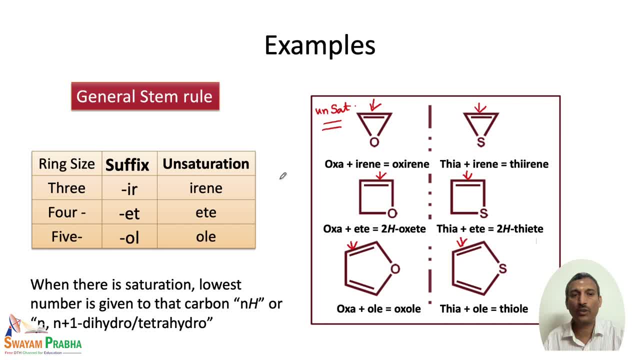 unsaturation. that means the name are going to be little bit different compared to the saturated one. so we have seen the suffix. will have to add ir, et and ol for three, four and five membered ring. so this is a three membered ring, so we have to add ir and the unsaturation whenever it is present, the whole. 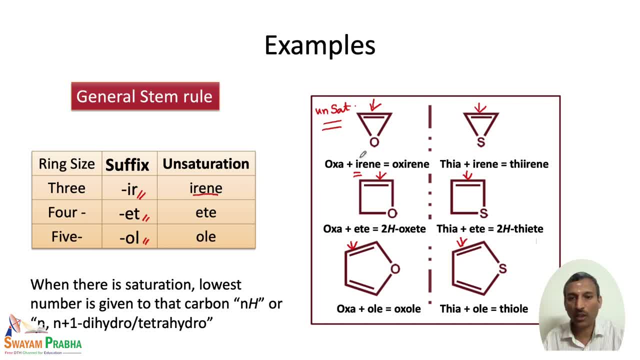 name is going to be irene. so that is what irene is the final name and avazia is the ring system, because whenever oxygen is present we give the prefix oxo to that particular ring naming. So oxo for oxygen. for sulfur we have thia. So that means when we talk about the 3 membered ring, I 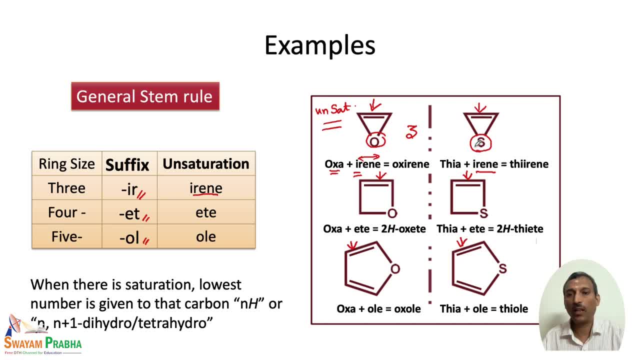 R E N. E is the stem ending and whether it is oxygen or sulfur. depending on that, we add the prefix oxo or thia, and when we combine these 2 things the last letter A is actually lost. So when we give the name final name, oxoirene is written as oxirene and thiairene. 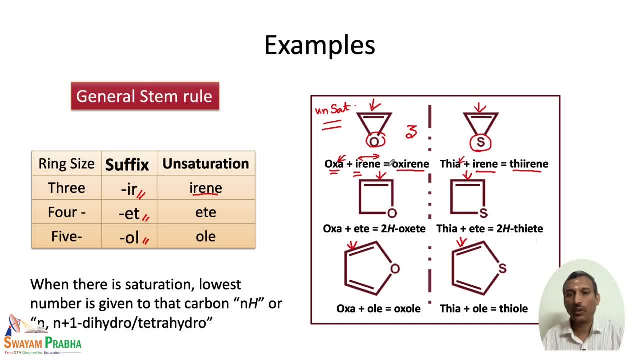 is written as thirene, So the last letter A is lost while we are writing this final name. Similarly, when we talk about the 4 membered ring, The four-membered suffix is ET and unsaturation is ETE, So oxo- ETE is the one we wrote. the 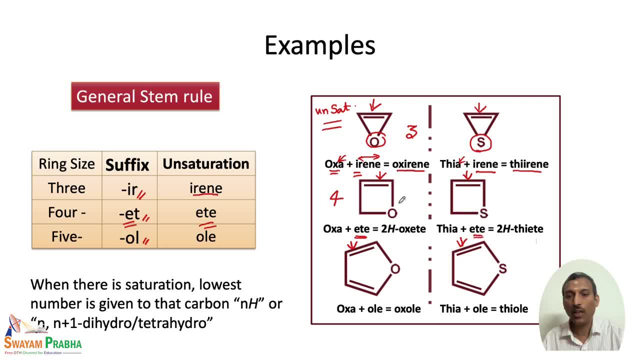 same way. thia ETE is the name we wrote, but we have one saturated carbon here. That means there is a 2 hydrogens are present here. So this is the third rule which we are going to add. That means, along with the saturation. 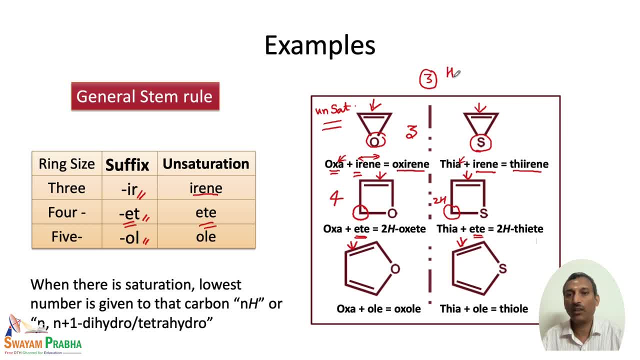 and unsaturation- saturation- we also have to mention the hydrogen. so this is the important rule: whenever there is a saturation, the lowest number is given that hydrogen as nh. so if we name this particular ring, the naming will or the numbering will start from here. this is number lowest number is given. 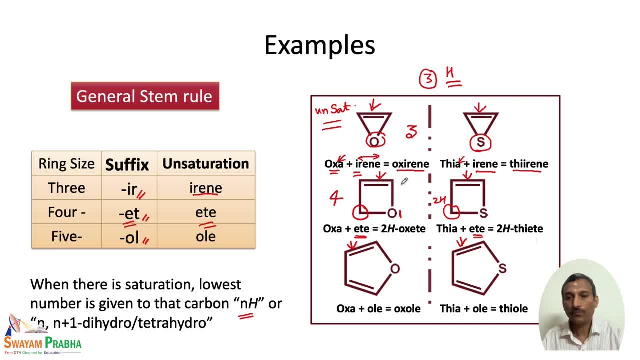 to the heteroatom 1 and of course in normal IUPAC nomenclature we give the next priority or the lowest numbering to the double bond. but in the case of heterocyclic compounds we are not going to name that this as that number 2, but the lowest number is given to the saturated carbon. 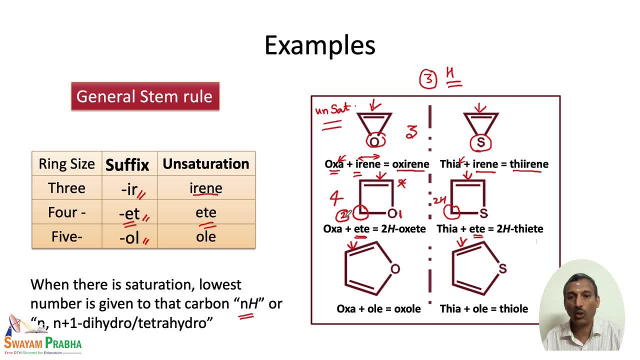 which is having two hydrogen atoms. so this has to have the lowest number and not the double bond. so when we number this here, we start number 1, this is number 2, this is number 3 and this is number 4. so in this particular case we have to have the lowest numbering to the double bond. so this is. 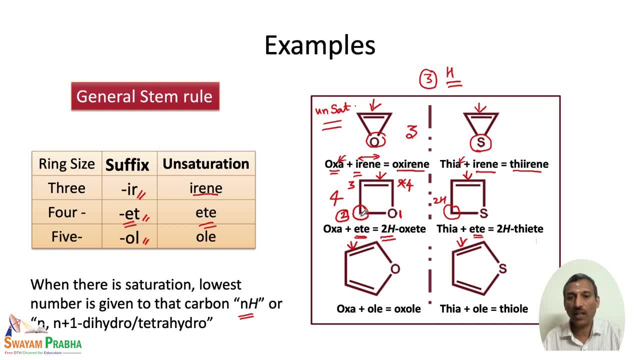 number 4, this is number 5 and this is number 6, so this is number 6 and in that particular case, the two position is having the hydrogen extra. so that is why we say 2h, o, e, e, o, x, e, t, e. oxa means. 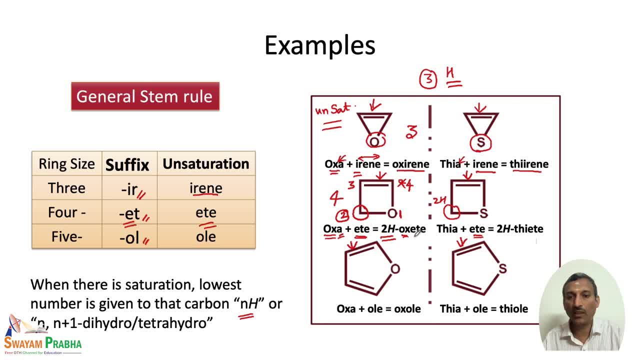 this is oxygen heterocycle. the last letter a is lost, so ox is added as a prefix, e, t, e is the suffix, so the name for this compound is 2h oxide, and when it is a sulfur, the same thing. we are going replace that with the Thaya and the numbering again: here is the lowest number 1, this is: 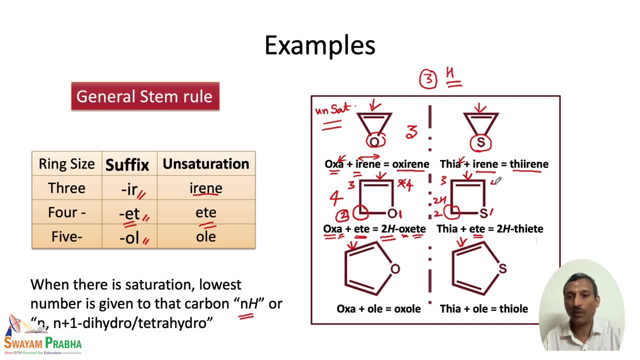 number 2 and this is number 3 and this is number 4.. So when it is a 4-membered ring, the suffix ending is ETE, and the sulfur is present, Thaya, and in 2 carbon it is a saturated. 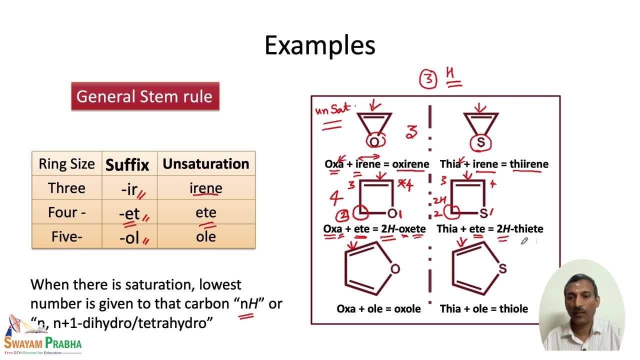 carbon. So we have to add the 2H here. So this is 2H Thayit. And when we talk about the 5-membered ring, so the 5-membered ring's suffix is OL and the unsaturation is OLE, So the ending is going to be OLE. We have an oxygen, so this: 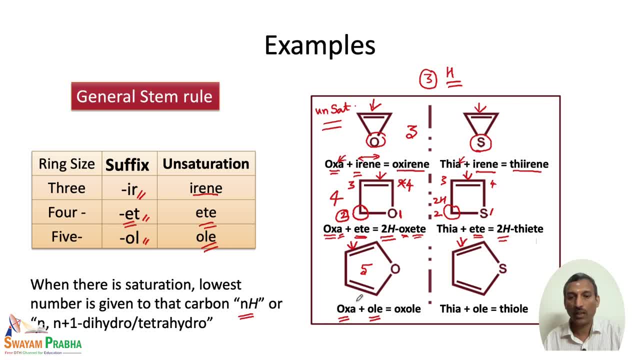 is OXA, So OXA plus OL, and the last letter A is last, so OXOLE. So this compound is nothing but OXOLE according to Hans Wildemann nomenclature. Hans Wildemann nomenclature, And when we talk about the next one, which is the 5-membered ring. so here again the 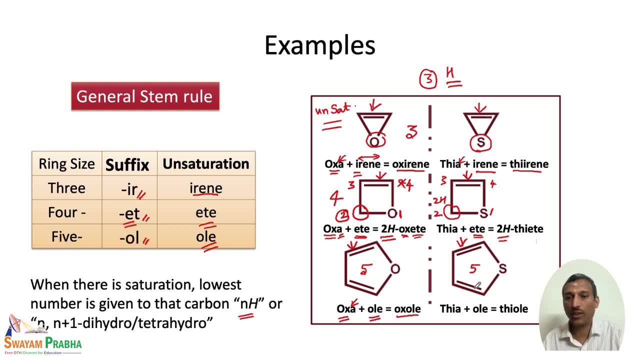 number. there is no saturated carbon, like the case of 4-membered ring. So that is the reason this can be given like a normal suffix, and the unsaturation because we have 2 double bonds. So Thaya, OLE and Thayole, that is the name which is given for this particular. 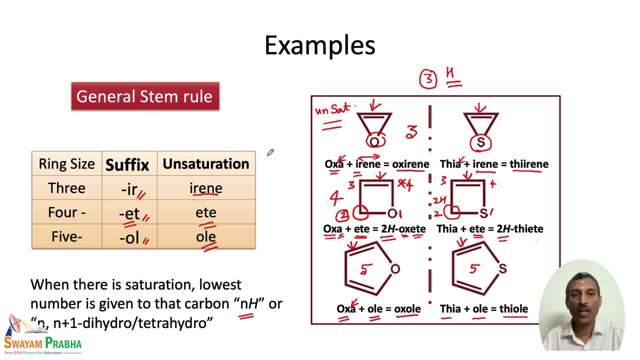 compound. So this is the general stem rule and in this particular case we talked about all the unsaturated compound. That means at least one double bond is present in these particular systems. So even if we have a double bond when there is a saturated carbon with 2 hydrogen atoms, 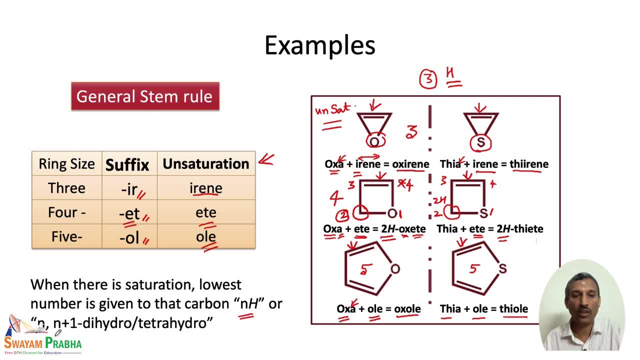 they are actually given the number, like NH or NN plus 1 di-hydro, tetra hydro, depending on the size of the ring, we can actually add these kind of prefixes. So when we give the numbering, the hydrogen atom, which is the saturated carbon, always gets the lowest number. So this: 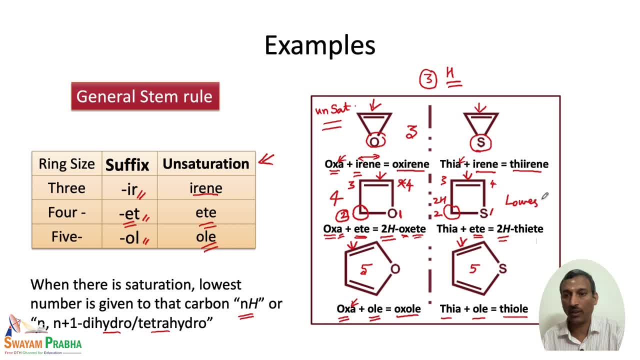 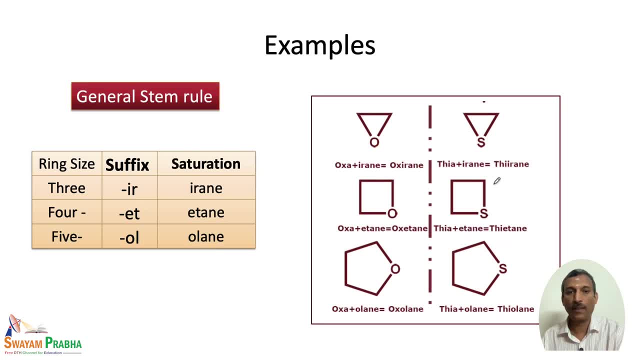 is one thing you have to remember: the lowest number for the hydrogen atom or the saturated carbon. Now we are going to the saturated system. So in this particular saturated system, we do not have any double bonds. We are not having any double bonds. So here the saturation. 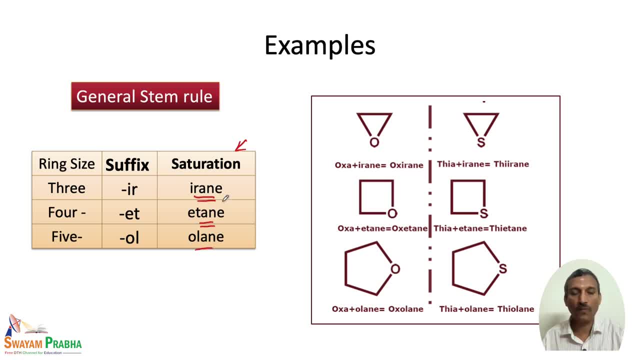 means the ending only changes. So in the previous case we have irin, Here it is irane. So oxo is the oxygen heterocycle and irane is the name. So when we combine these two, the last letter A is lost, so oxyrene. So this three membered heterocycle is called oxyrene, And 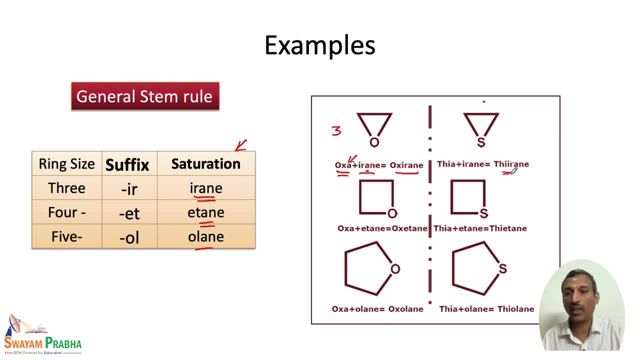 if it is a three member sulfur heterocycle that is called thyrane, And if it is a four membered heterocycle with oxygen, then the ending is etane, oxoetane, So oxetane, and if it is thia, it is thia etane. 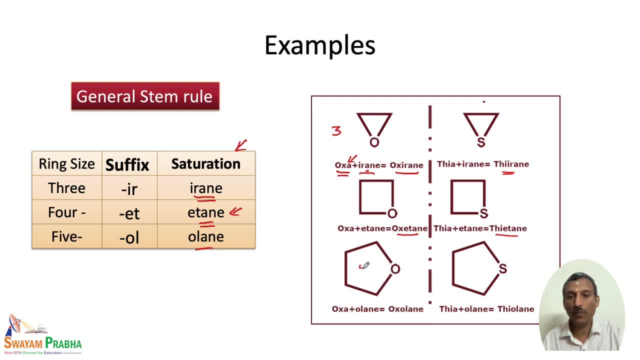 thietane, and if it is a 5 membered ring, the saturation is olane, So oxo plus olane oxolane. and if it is a sulfur, it is thia plus olane thiolane. So this is how we actually have to. 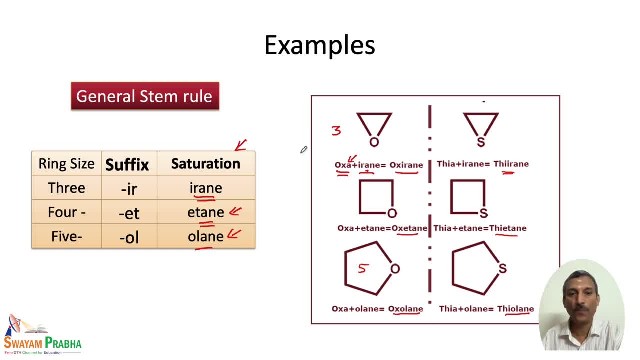 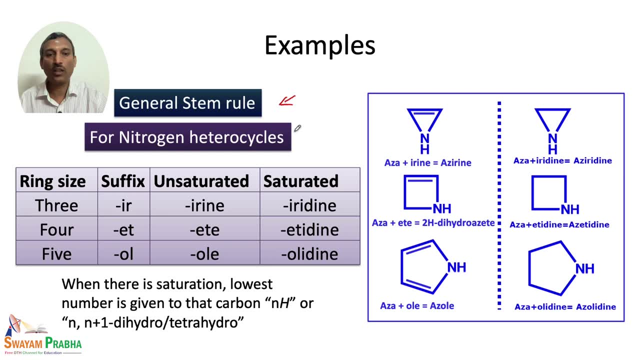 give the heterocyclic compounds nomenclature. The major difference comes in the case of nitrogen heterocycles. So here the rules are little bit different. So we have two examples: one is a saturated one, another one is a. one is a unsaturated system, another one is a saturated. 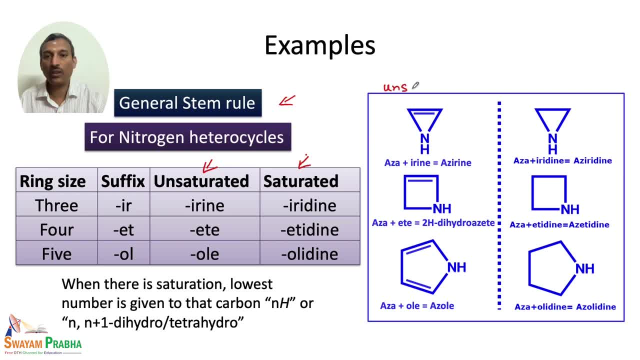 system. So this is the unsaturated one, this is a saturated one. so in the unsaturated one we have at least one double bond in the system. So we have to follow the same thing, what we have used earlier also. The only thing is this is the suffix with which. 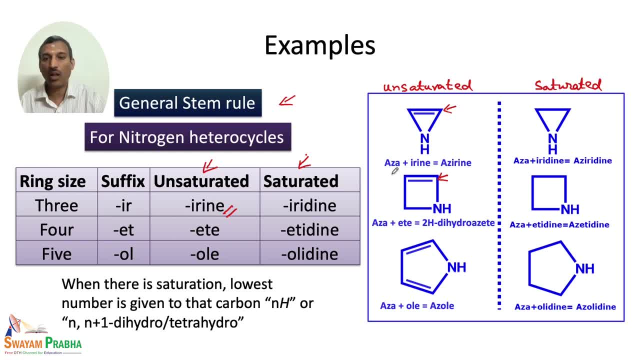 the name will end irin and aza is a nitrogen analog, So whenever we have a nitrogen heterocycle we use the prefix aza plus irin. as we know, the last letter, a, will be lost, so azirine, and if it is a saturated one, 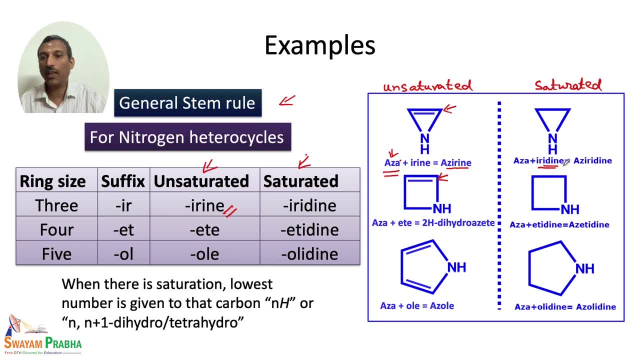 the name ending name is going to be iridine. aza plus iridine is aziridine. So this is a three-membered heterocycle with the nitrogen atom. So this is a saturated heterocycle and the name is aziridine. So this is how we can actually give the IUPAC nomenclature for the. 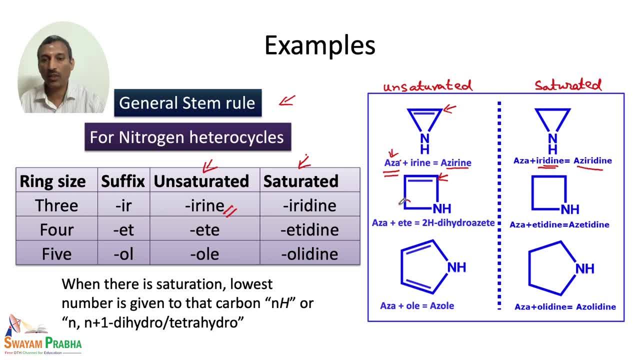 carbon. And when we talk about the four-membered ring, here again we have a saturated carbon, so that means the number has to be the lowest number has to be given here. so that is why we have the two-hich number given here, And in the case of completely saturated one we do not have this. 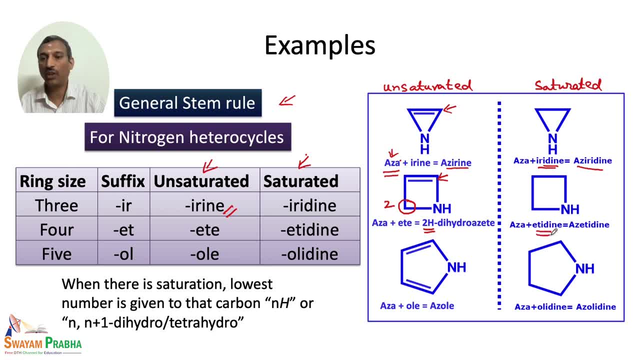 requirement. so that is the reason, only the ending changes. So aza plus etidine. acetidine is a four-membered ring and in the case of four-membered ring with one double bond it is two-hich dihydroacete. so that is what we have written earlier. also, whenever there is a heteroatom, we 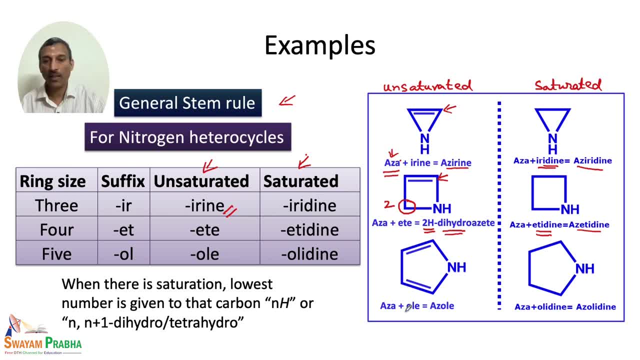 may have to write that as a dihydro system, And if it is a five-membered ring, which is an unsaturated one, we have azole, aza plus ole azole, and if it is a saturated one, aza plus oleidine. so the ending for the saturated system is oleidine. So azoleidine is the name for this. 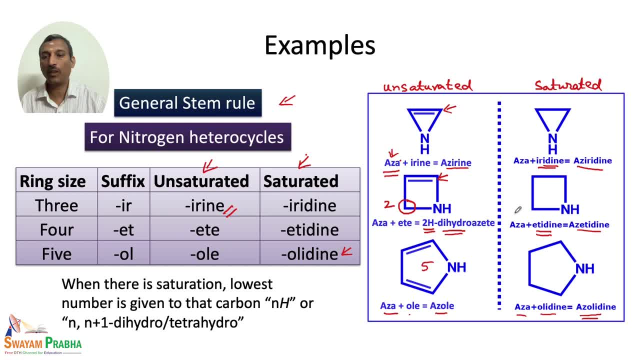 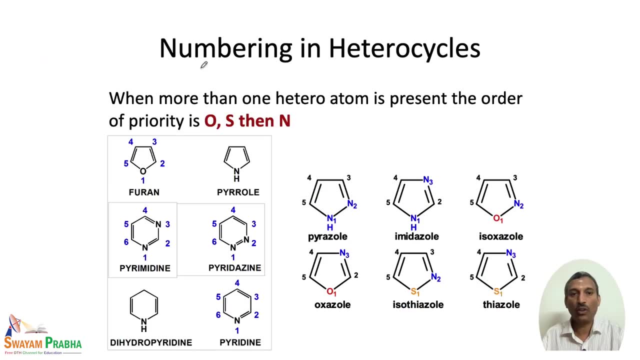 compound. these are IUPAC given nomenclatures. but but of course for all these simple compounds we also have common names and we will also be looking at what are the common names for all these compounds. So when we talk about the numbering, so the numbering of heterocycle, follow a little. 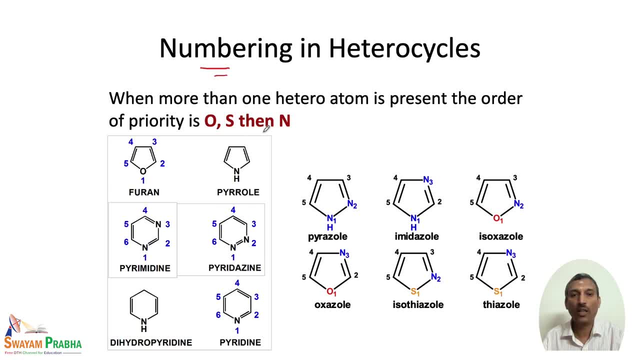 bit different rule compared to other cases. So in this particular case oxygen gets the highest priority. Priority is the numbering of oxygen. So in this particular case oxygen gets the highest. priority means it should get the lowest number and followed by sulfur and then finally by nitrogen. So there, 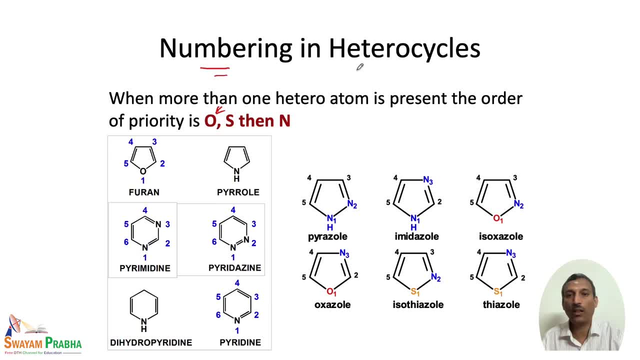 are two things you have to remember when we are naming a heterocycle. one is the basic name of the system and another one is the numbering. So these are two different things we have to remember. and when we talk about name, the nitrogen gets the priority, because whichever is the nitrogen, 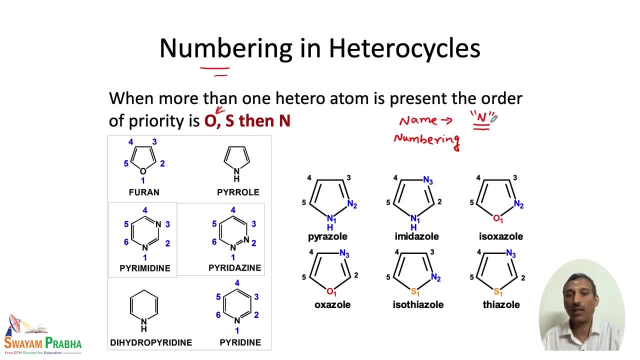 ring is given as the base ring and the name is given based on nitrogen only. So this is the highest priority for the name and when we talk about number, the number nitrogen does not get the highest priority, but nitrogen gets the least priority. oxygen gets the highest priority, followed by sulfur. 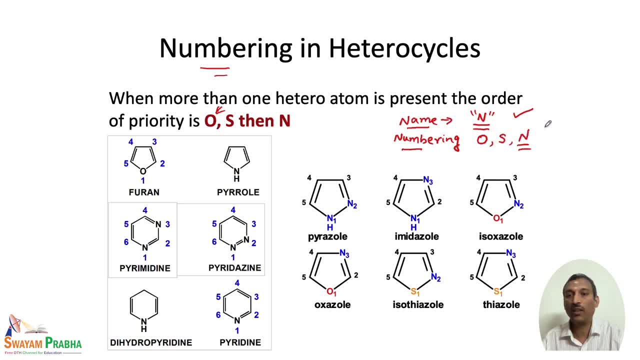 then only nitrogen is given the numbering. So these are all the two things you have to remember when we talk about heterocycle nomenclature. Say, if there is only one heteroatom, we have no problem, So we can give the lowest. 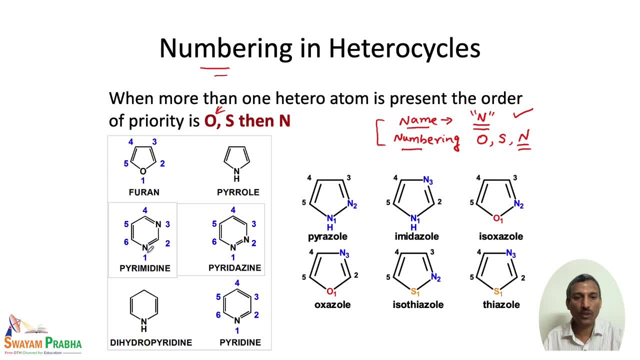 number to the heteroatom. When there are two heteroatoms we actually start from one of the heteroatom, then go to the next heteroatom in the shortest route. So for this compound we generally do not give the number as 1,, 2,, 3,, 4, 5.. So this is not a 1, 5 system. 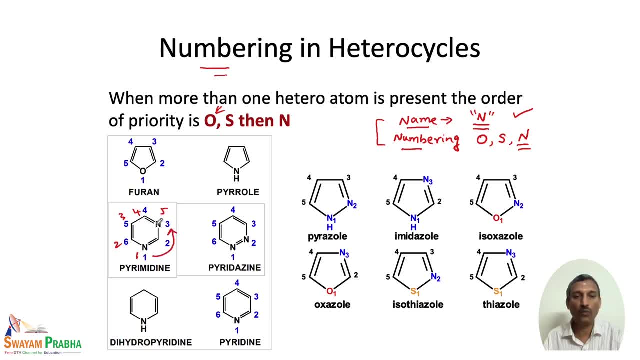 Usually this is a 1, 3 system because by this way only we get the lowest number for the second heteroatom, And when there are only one heteroatom, as I mentioned, we do not have to have any preference. We can always start with the lowest number with the heteroatom. 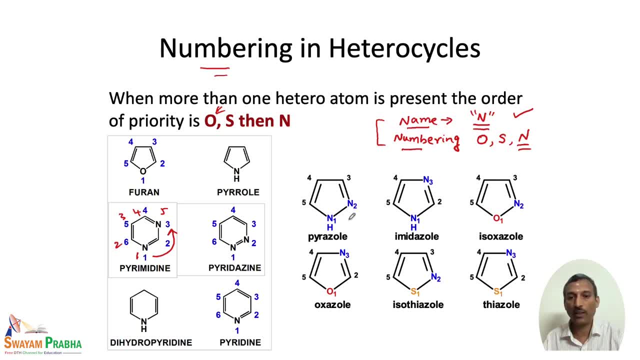 But when there are more than one heteroatom, as shown here on the right hand side, we have nitrogen 1, nitrogen 2. So these two are adjacent to each other, So we can give the numbering like 1 for this cell. 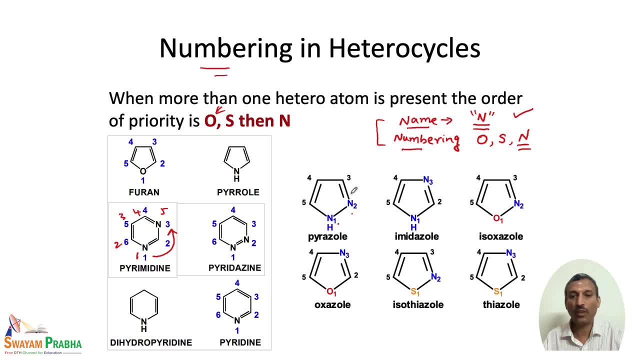 Saturated nitrogen, followed by the unsaturated nitrogen. So in most of the cases the hydrogen atom actually gets precedence. So that means when there are two nitrogens, one with hydrogen, one without the hydrogen, then which will get the lowest number is always the nitrogen. 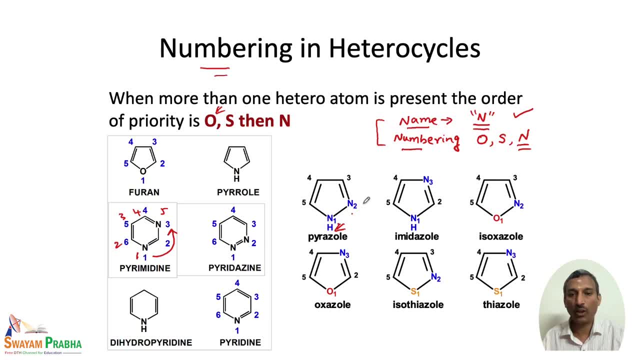 with the hydrogen gets the lowest number And this compound is not numbered as this as 1 and this as 2 is not the way of numbering. The nitrogen with hydrogen gets the lowest number, followed by the next nitrogen. So that is how the numbering is given for this system. Similarly, in this system also, this is not. 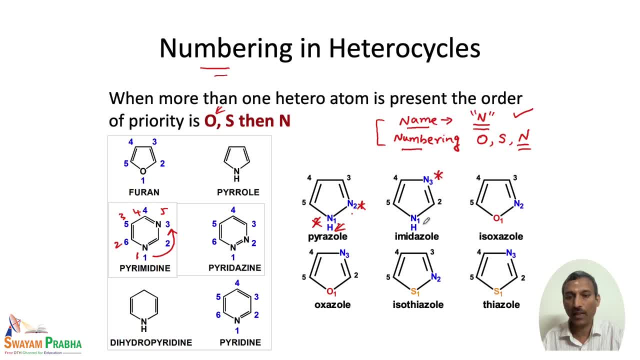 numbered as 1.. Only this nitrogen with hydrogen is numbered as 1, and this nitrogen gets the number 3.. So this is how the numbering is actually given. when there are more than one hetero cycle, one heteroatom is present in the system And when there is between oxygen. 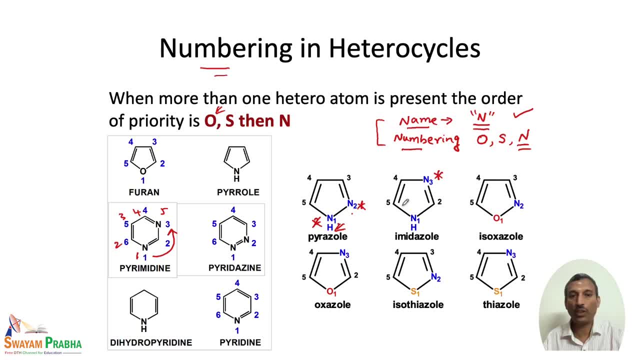 and nitrogen. as we see, oxygen gets the lowest number, So this will start from number: oxygen on number 1, nitrogen gets the number 2 and the same is applicable here also. So this compound is called isoxazole and this is called oxazole. These are common names and we will 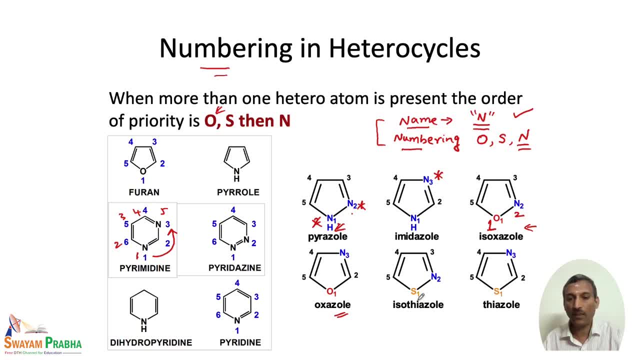 look at these things a little later. And when there is a sulfur and nitrogen, again sulfur gets the priority in getting the lowest number, followed by nitrogen. So when we number the heterocycles, heteroatoms, we have to follow. oxygen gets the highest priority. In other 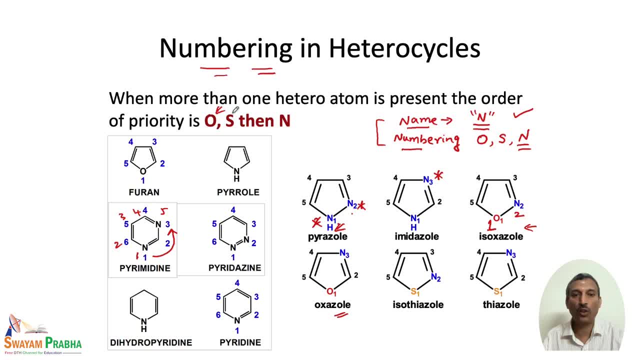 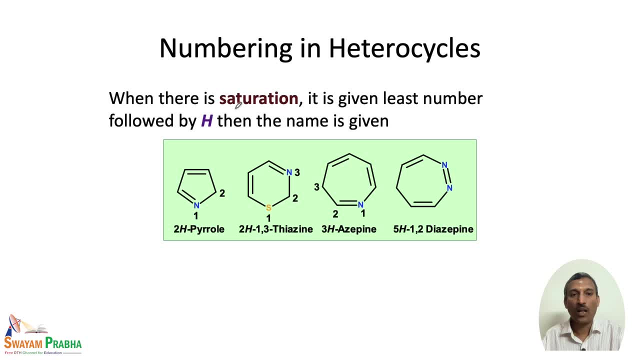 words, the lowest number is given to oxygen, followed by sulfur, then only nitrogen gets the number. So this rule. we have actually seen the numbering of saturation, So we have to apply. the lowest number for this saturation point is a saturated carbon. that saturated carbon is given the lowest number, unlike the normal. 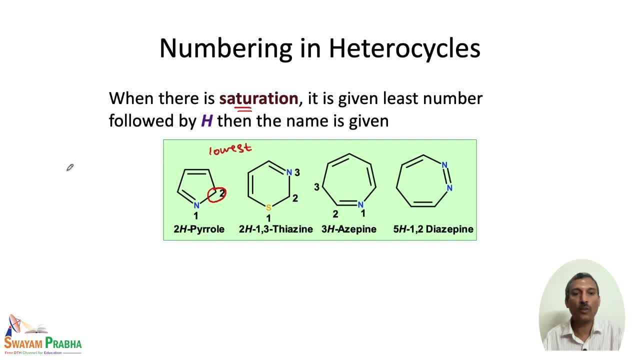 iupac nomenclature. in the case of iupac nomenclature, if we have alkane and alkene, we generally give the preference to the alkene carbon. so the alkene carbon gets the lowest number, followed by the alkane, whereas in the case of heterocyclic nomenclature it is the saturated 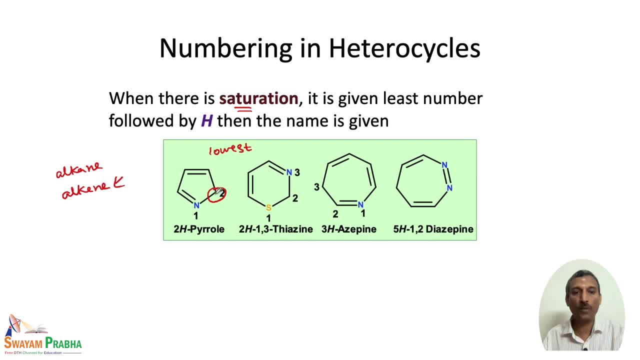 carbon with the hydrogen atom, gets the lowest number. so that is the reason this is called the 2h pyrrole, and if we have to give the lowest number to the double bond, then we can actually start from the other way around. so one, two, three, four and this carbon will become the fifth one. 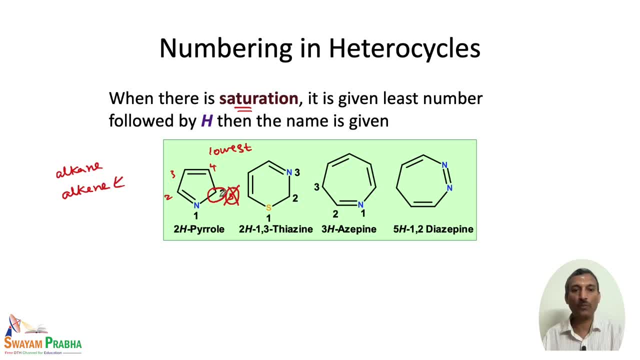 so we are not giving the phi number to this particular carbon, but we are giving number two, that is, the lowest number is given to this saturated carbon. similarly, when we take this thiazine unit, this carbon is the saturated one having the lowest number and, again, priority. as you know, sulfur gets the highest priority, getting the lowest number. 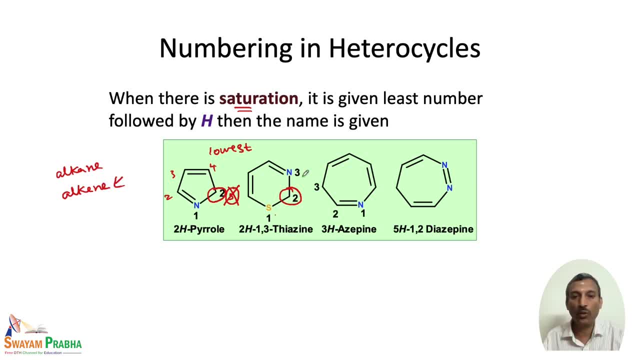 followed by nitrogen. so that's the reason. this is one, two, three and in the case of acipene, this carbon is having the lowest number. similarly, for this one, how to number? we can start from here, and this is the fifth one. if you move from the other direction, let us stay from here. one, two, three. 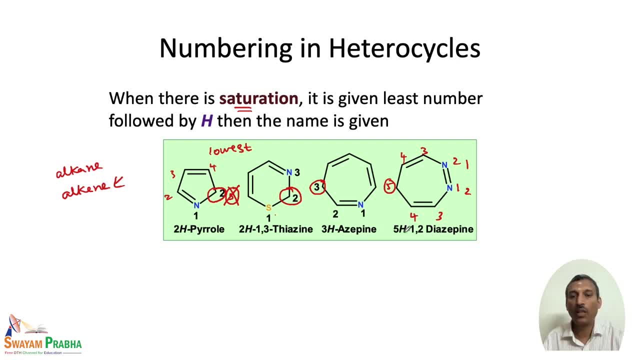 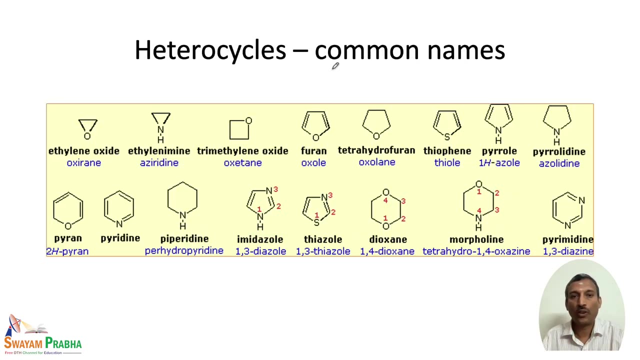 four and five. in both the cases this is the lowest number. so this compound is given as 5h12 diazepine because nitrogen is present in one and two positions. so that is what one and two diazepine is, the seven membered rings name. so, as we mentioned, there are lots of common names which 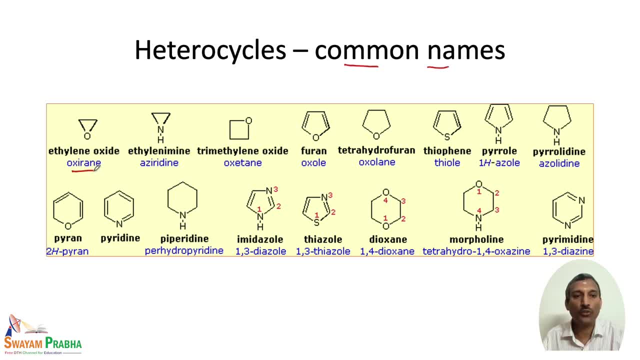 are used in heterocycles. we know the name oxirin is for this three-membered oxygen heterocycle, but this is generally called as ethylene oxide, and acyridine is another name given and ethylenamine. ethylenamine is the name for this particular cyclic system and, of course, furon is a common 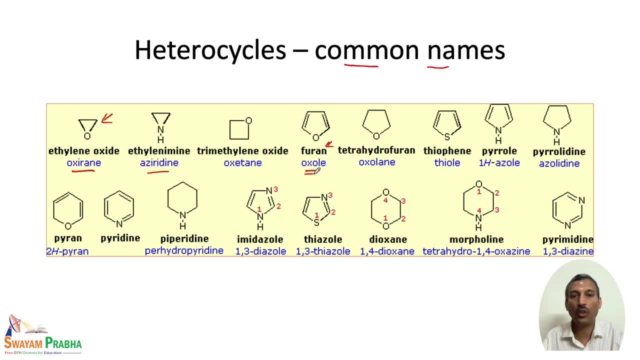 name which many people are aware of, and oxal is the name for iupac nomenclature. similarly, oxaline is not generally used, whereas tetrahydrofurane is the name which is commonly used in synthetic chemistry and heterocyclic chemistry also. similarly, thiophene, pyrrole, pyrrolidine are the names which are generally used, even for 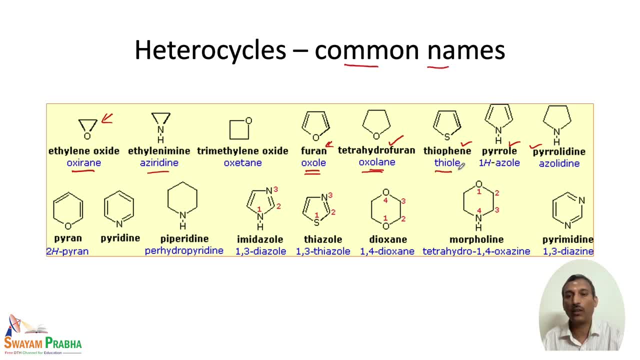 many of the nomenclatures, although iupac nomenclature gives a little bit different name. but these iupac nomenclatures are not commonly used for these kind of simple systems. for example, pyridine is same whether it is iupac nomenclature or the 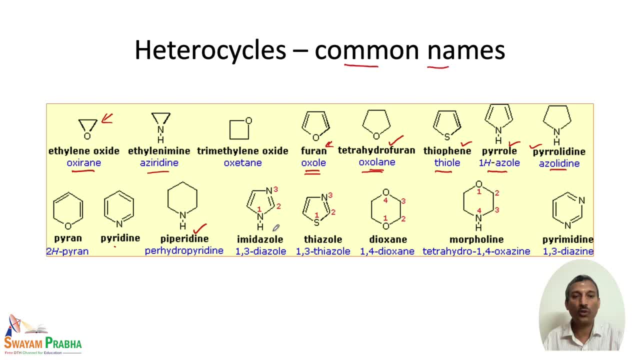 common name piperidine is the one which we generally use: imidazole, thiazole, dioxane or morpholine pyrimidine. these are all the common names which are used for various heterocycles. of course the iupac nomenclature are given below, but these are not regularly used. 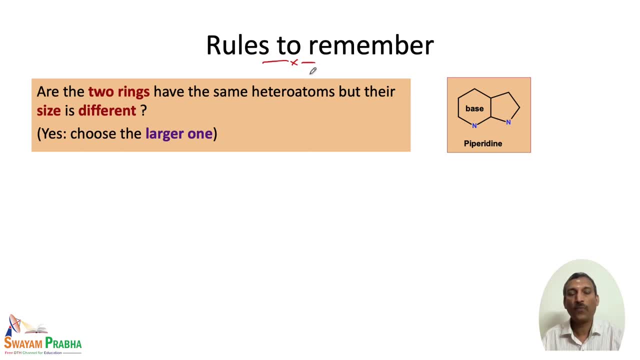 so let us look at some of the important rules for naming when there are more than one heterocyclic ring, say, for example, if there are two rings are present and if both of the rings are having the same heteroatom but their sizes are different. so how do we name that compound? so the answer is we. 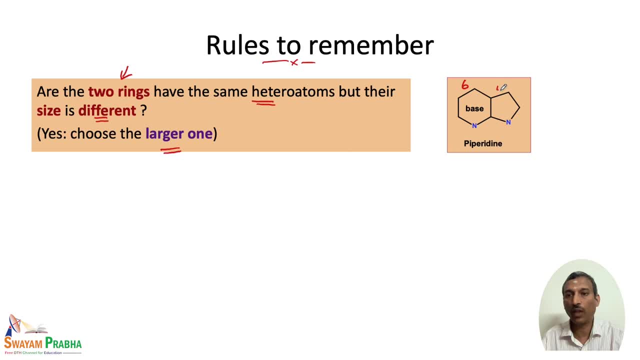 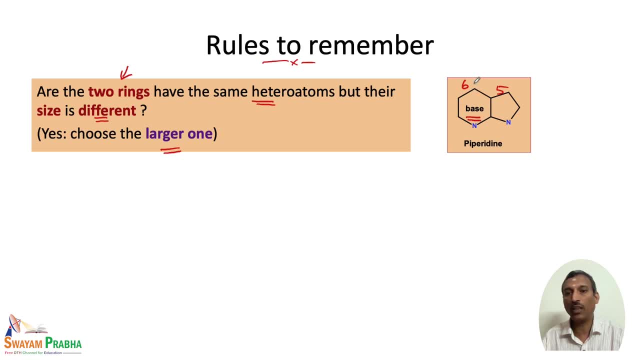 based on the six membered ring only because this is the larger ring, so we have to follow the name. that means the ending is going to be on piperidine structure. that means this compound is named as a piperidine derivative and not the five membered ring derivative. so this is one rule we have to. 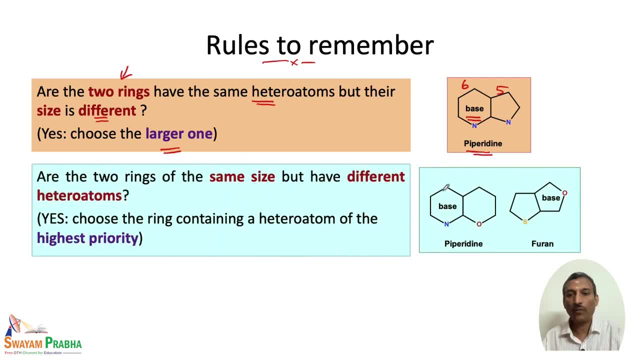 remember- and if we have two rings which are having the same size but the heteroatoms are different- say, for example, we have the nitrogen and oxygen. so the rule is basically, whenever we have two different systems, if they have the same size, then, depending on the heteroatom, we are going. 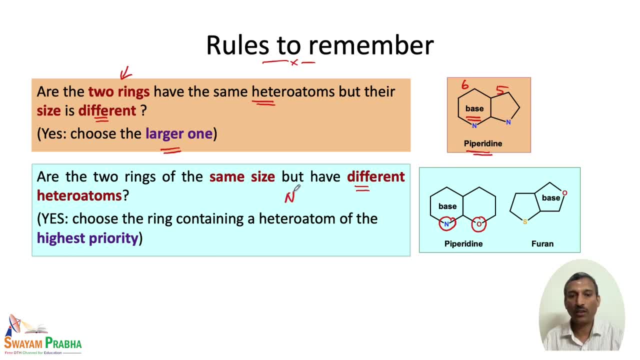 to number. so the priority is nitrogen is getting the highest priority for this naming. so the name follows nitrogen, oxygen and sulfur rule. so that means whichever is the nitrogen heterocycle that is named as the base ring. that means this compound is named as a piperidine derivative and not the oxygen derivative. similarly, when we have oxygen and sulfur, this is a. 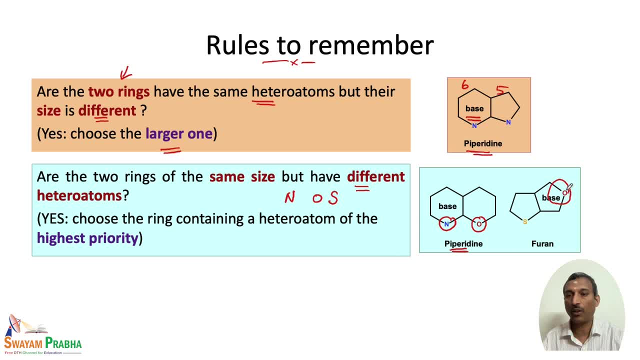 five membered ring where oxygen has the priority. so this is named as a furon derivative and not as the thiophene derivative. so let us recap the two rules: when the ring sizes are different, the bigger ring gets the base unit. when the rings are of same size but the heteroatoms are different, 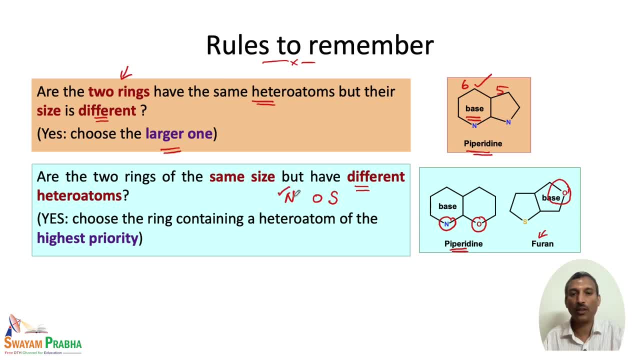 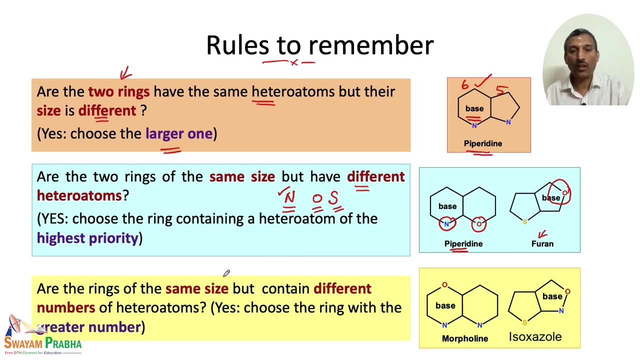 then the rule is nitrogen gets the highest priority. that means the base name is given using nitrogen heterocycle, followed by oxygen. then only sulfur is given, and if there are having the same size but the number of heteroatoms are different, this is very easy to understand. 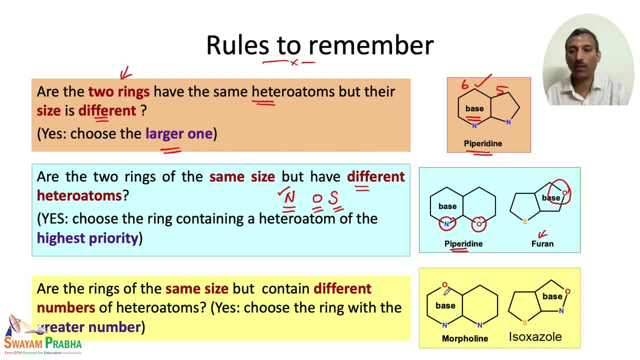 answer because when there are more than one hetero atom, then obviously that ring is going to get the base name. so when there are nitrogen and oxygen in one ring and nitrogen only in the other ring, the name is given based on the two hetero atoms present in one ring. that means it is going to 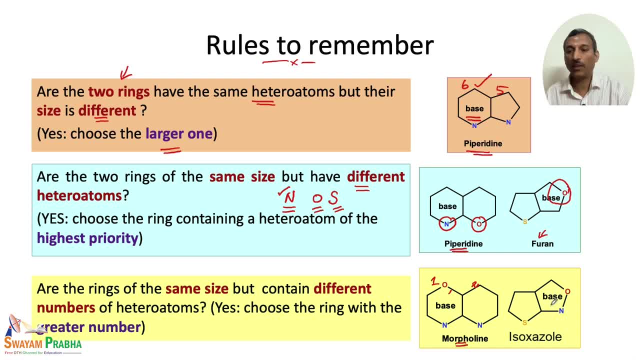 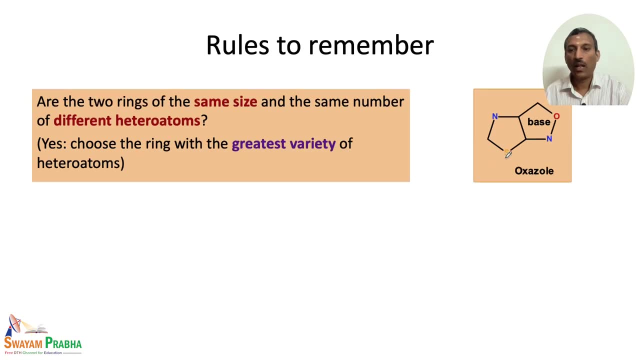 be named as a morpholine derivative, and similarly when we have the nitrogen and oxygen. so this is basically the isoxazole derivative. so this compound is going to be named as a isoxazole derivative and if the two rings are of the same size but the number of hetero atoms, that means 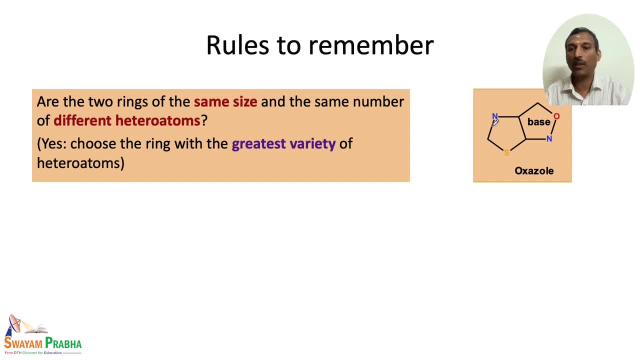 the two hetero atoms are also same. but if they are different, then how are we going to give? the greatest variety is the one by which we are going to number it. so that means here we have nitrogen and sulfur. in this case we have nitrogen and oxygen, so the nitrogen and oxygen gets the highest priority. 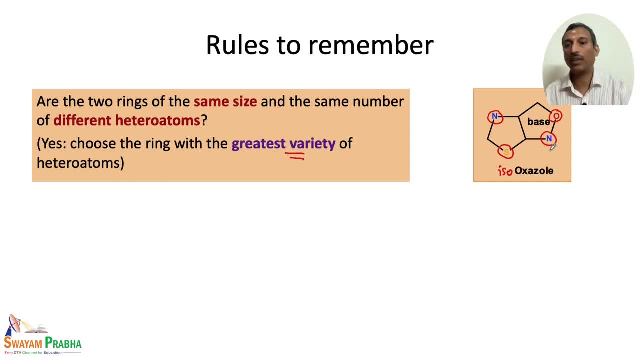 so this is isoxazole derivative. so we are going to name this as a isoxazole derivative. so here oxygen gets the priority compared to sulfur. both other units are similarly same compound. that means nitrogen is the same. so we can ignore that and we have to go for the 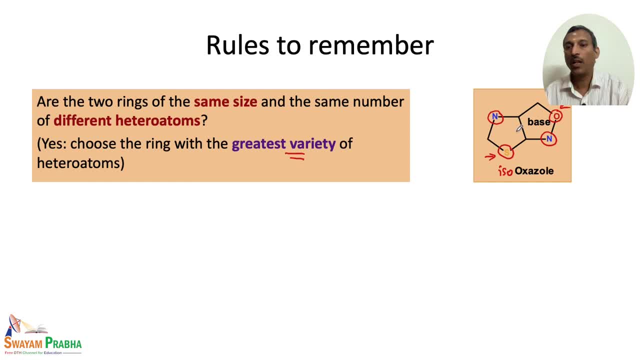 next hetero atom, which is having the highest priority. based on that, the number of hetero atoms are named as water. so this is how we get the highest priority and that best number of variation over time, and this is the cause for the change. and so how do we pick up a number which is top priority? 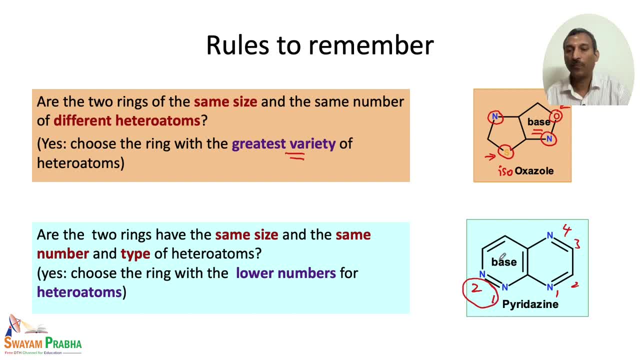 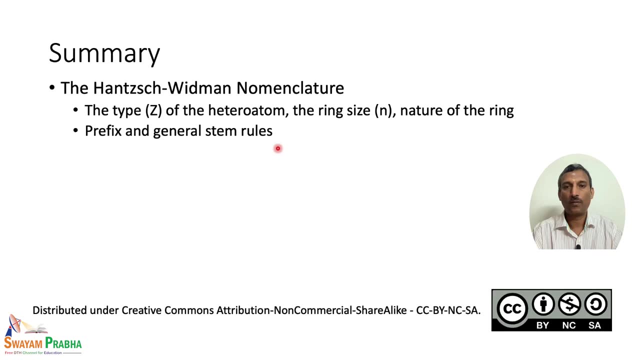 so these individuals. as shown on the screen is an Crowes circle. this is another information. Natasha- is the reason the base unit given is the pyridazine unit for this kind of compound. So these are all the ways by which we can actually name various heterocycles. Let us recap in the summary what 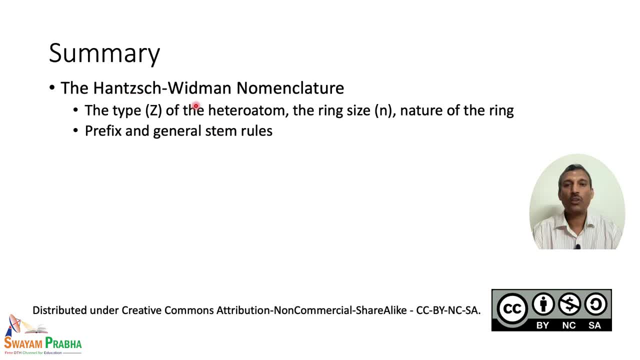 we have studied so far. We have studied about Hans Widmann nomenclature. So here we studied about the type of the heteroatom. that means based on nitrogen oxygen or sulfur heterocycle. How a hetero cyclic ring is named, we have seen. When it is an oxygen we use oxa, when it is a 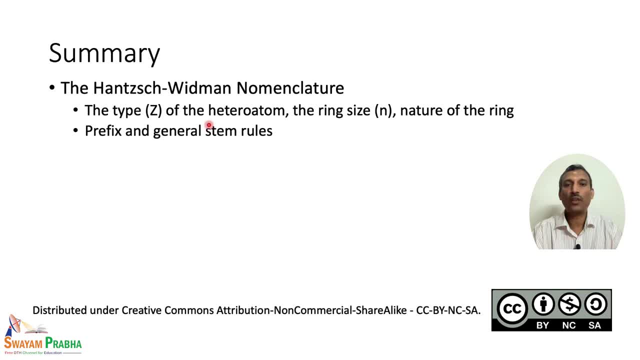 sulfur, we use thia and when it is nitrogen we use asa as the prefix for naming. We also studied about the ring size, the nature of the ring, the numbering for each heteroatom, all those things we have seen. We have also studied about, if there are more than one ring, how to name which ring. 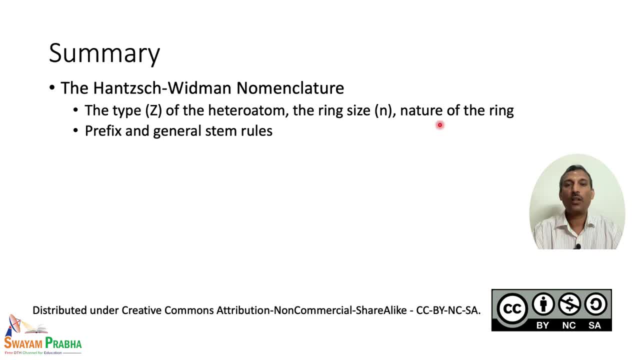 is going to be considered as a base ring and, depending on the saturation, how we are going to name the ring. We have also studied about the numbering of the ring, the numbering of the ring, heterocycles- all those things we have studied. we also studied about the 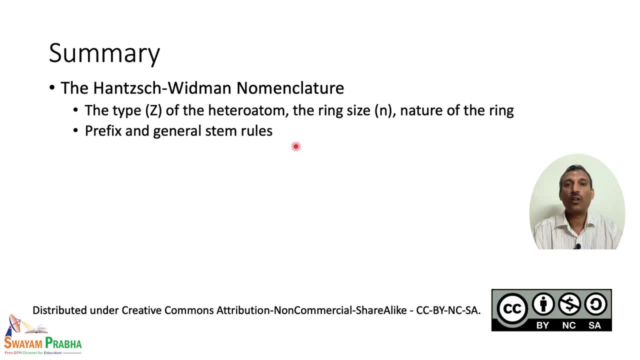 prefix and the general stem rule. what are the different ways by which the hetero cyclic compounds are named that we have seen, starting from three member to nine membered. we have compared how nitrogen based hetero cycle and hetero cycle without nitrogen are named. we have seen whether there is a saturation.